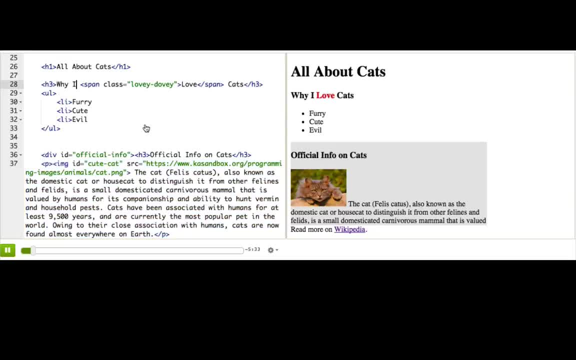 this paragraph is a box. even the span that we made is a box. Some of the boxes are big, some are small, some are inline, like the span, some are block, like the div, but they're all considered boxes. Why does this matter? Because it's something called the box model, which you 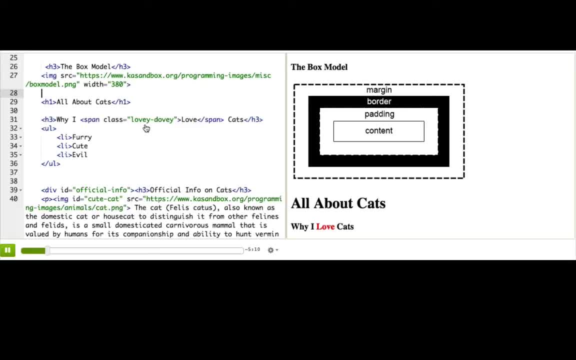 can see in the diagram I just pasted in, Every element's box has four parts: the actual content, the padding, the border and the margin. We can use CSS to modify the padding, border and margin. so you'll understand soon. 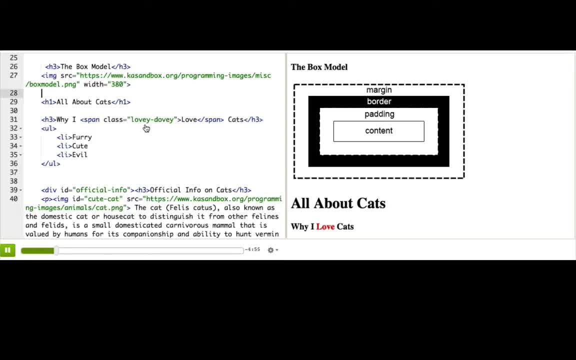 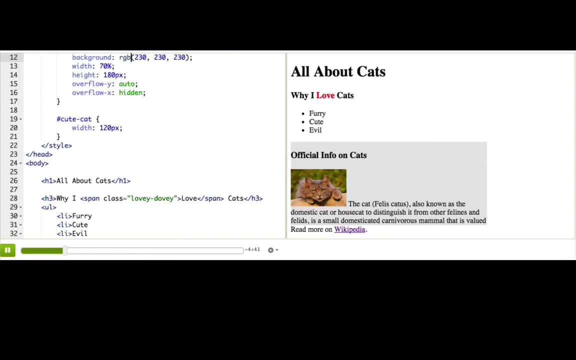 Let's start with the margin. That's the transparent area around the box that separates the box from other elements. We'll specify margin using our favorite unit pixels To add 15 pixels of margin on every side of the official info box. we can just write margin 15px. See the change that made. 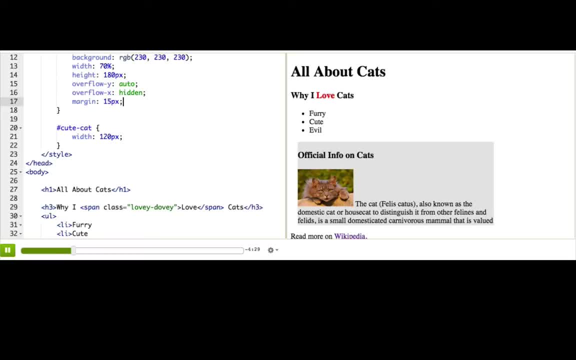 What if we want a different amount of margin on each side? For example, as you can see in the diagram, margin 15px is equal to margin 19.. We can write some margin on the top, bottom and bottom, like more on the top, bottom than the left-right. 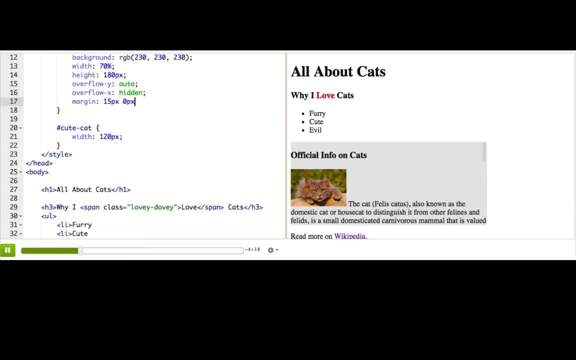 We can write those amounts in clockwise order, starting from the top. So top 15px, right, zero px. bottom 10px, left, 6px. Or we can use specific properties for each side if we only want to specify a few sides, Like if we want to have some space around the cat picture on the right and then 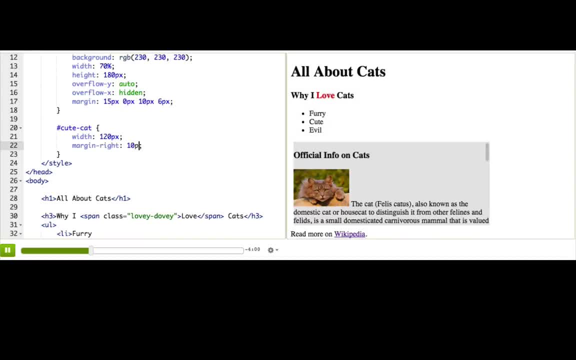 each box should be a number. then we can use some more margin. We can say margin 15px for that, and then we can say margin 15px for that and then add some more margin, and then we can write again margin 15px. See the change in the search box. Now let's say margin 15px is equal to margin 19,. 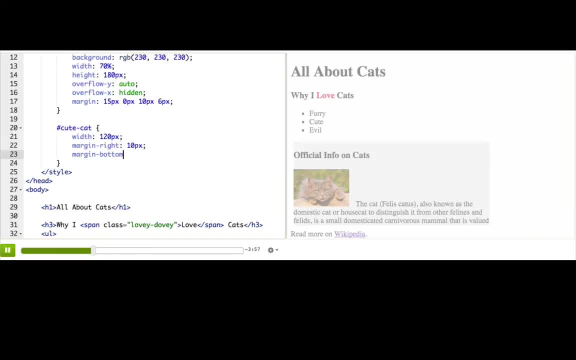 and then we also just want some on the bottom and we're happy to have the default margin for the other sides. There's also a special value for margin that will help us do something fancy with our pages. To show you that, I'm going to add a div. 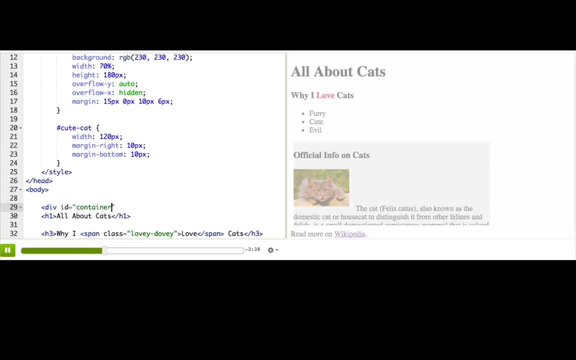 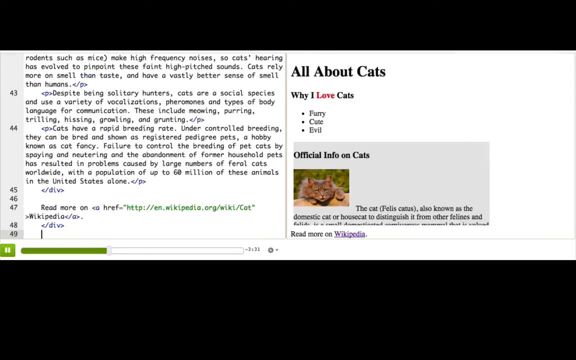 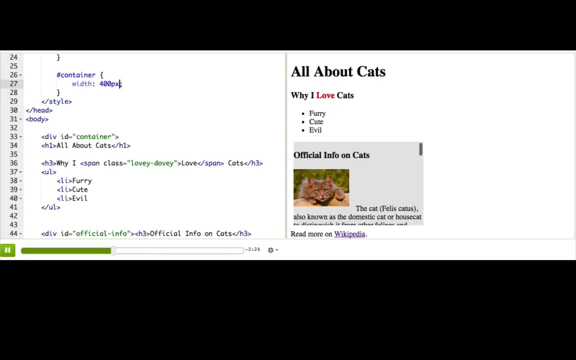 around the entire page, give it an ID of container. Let's put this tag here, so it contains everything. Now I'm going to add a rule for that div to give it a width of 400px, and I want to center it on the page. 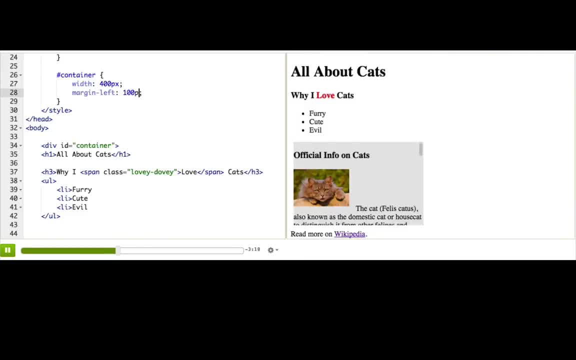 I could specify a margin left 100px, because that looks centered to me but it may not look centered to you, because your browser might be bigger or smaller. What we want is to be able to say: give it however much margin it needs. 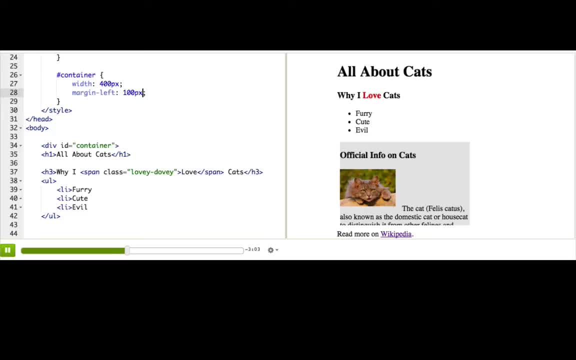 so that it's got equal margin on both sides. That is exactly what we want. That is exactly what margin-auto does, and it's a great way to center divs on a page. Now that we've centered that div, we might want to make it even more distinct. 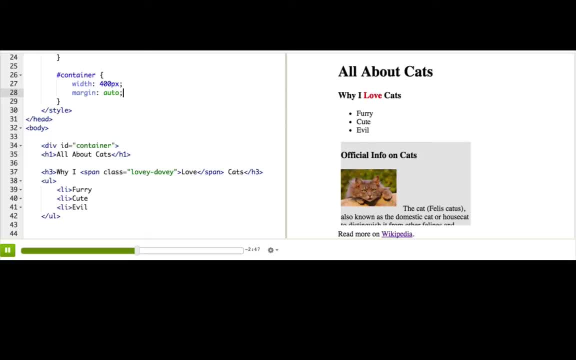 by adding a border around the edge of it using the CSS border property. Let's add a red border to that div. We type border and then we need to specify three aspects of the border: thickness, style and color. For a thin border, we can just type onepx. 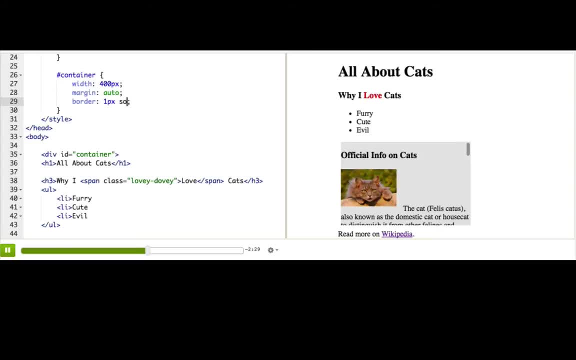 For a solid line, nothing fancy, we'll just type solid And to make it red, I'll pop in my RGB color picker and pick a nice fiery red. Okay, Just like with margin, we can specify the border for just one side. 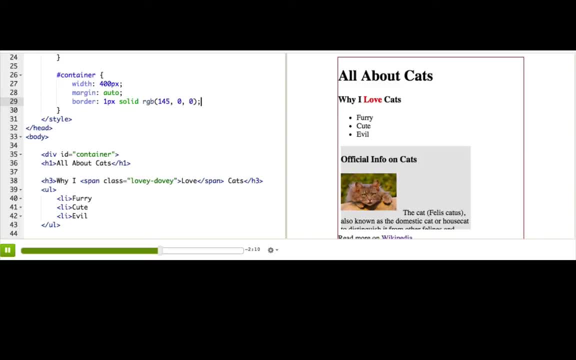 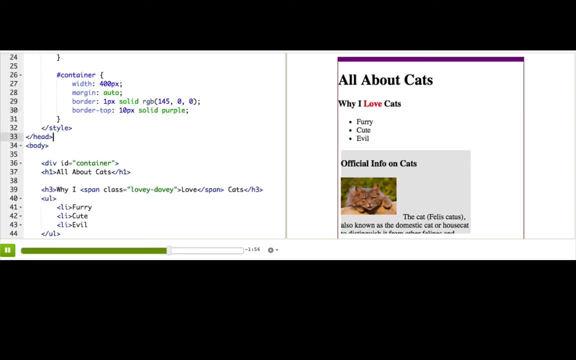 Like, if we want a really thick purple border on the top, we'll add another property: Border top- 10px solid. Border top- 10px solid- Purple. Cool, Now let's add a frame to the image and play around with border styles. 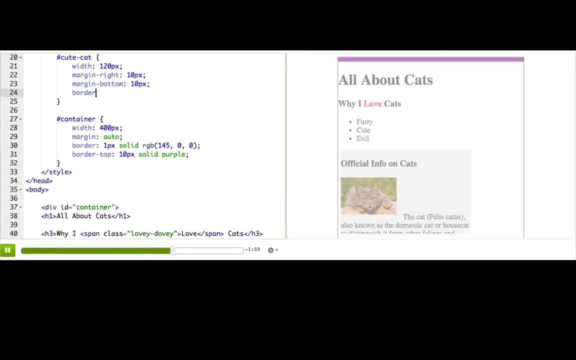 Going up to our cute cat. Let's see border 6px. Let's try groove red. Okay, no, no, I don't like groove. Let's try double. Eh, let's try ridge. Aha, now that looks like a frame. 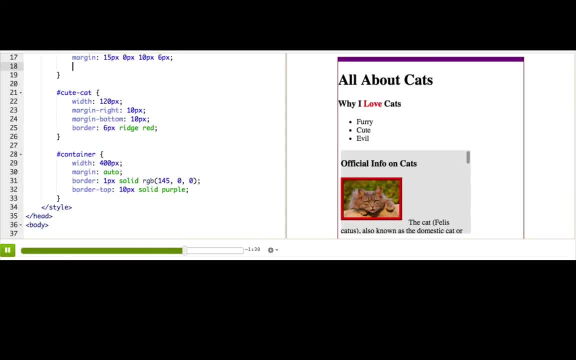 Okay, Let's add a border around our official info. Let's see border. let's not make it too big: two pixels. Let's try dotted, and then let's pick just a subtle gray. Let me try dashed instead. Okay, that's what I want. 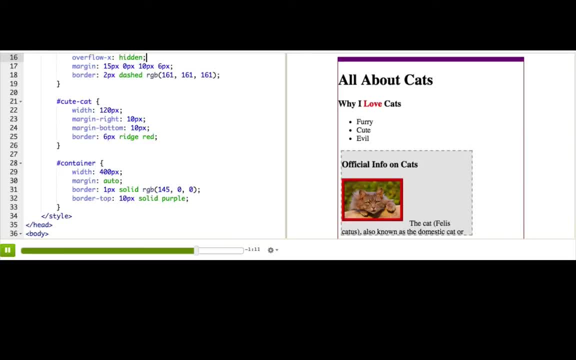 Now, with all these borders, something is bothering me a little. Actually, something's bothering me a lot. See how the text is budding up next to the border in the container And and budding against the text in the official info. That's so gross looking.